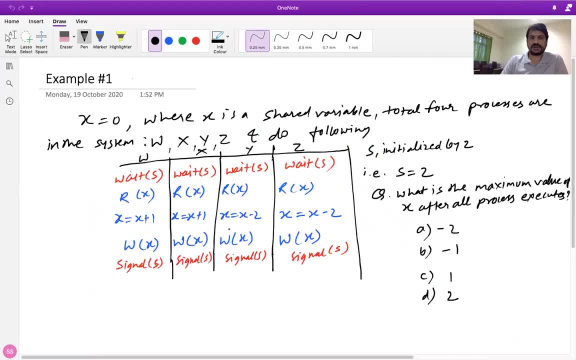 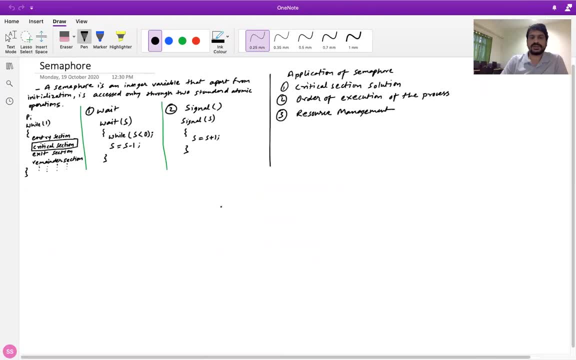 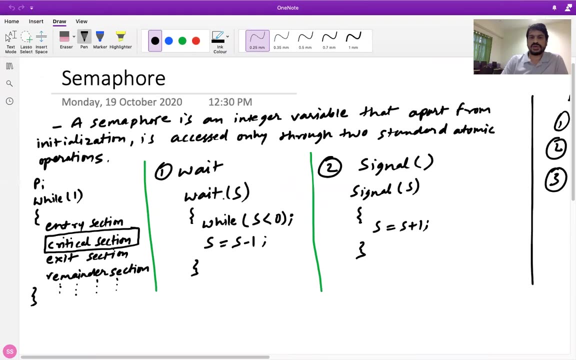 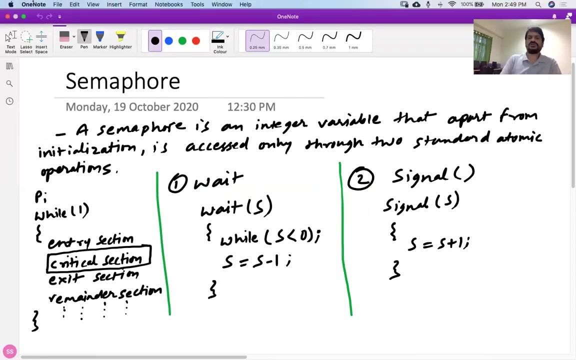 another separate topic of process synchronization and critical section is the topic called semaphore. now, what is a semaphore and why we required now till now what we have seen? we have seen different solutions. we have seen some hard software solution which was features and solution, and there is a 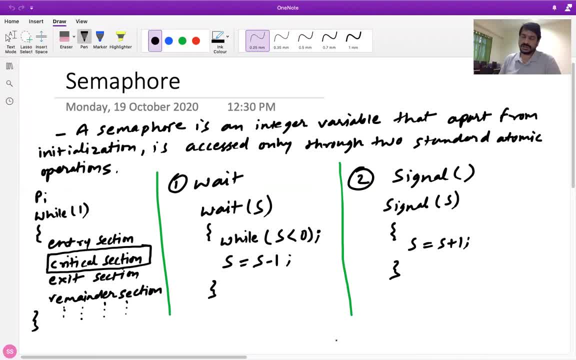 restriction of two process, that that solution is only for two process. now in the hardware solution we have seen test and wait, which is a complete solution, but again we have another solution called swap instruction, which is not a complete solution, which actually is having mutual exclusion but doesn't have the progress as well as the 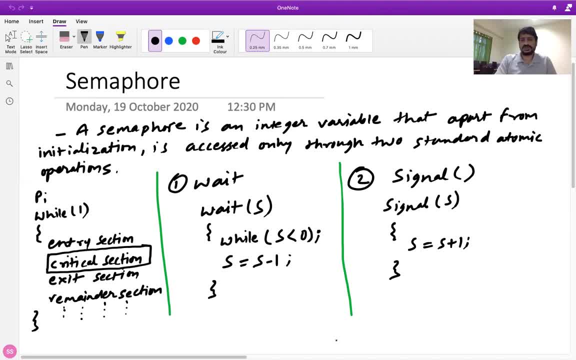 boundary weight, and that was again a hardware solution. now do we have any provision which will make as a software solution, for an number of processes means more than two processes. so the answer is yes. we have a solution which is called semaphore, and semaphore is used for the critical section problem and 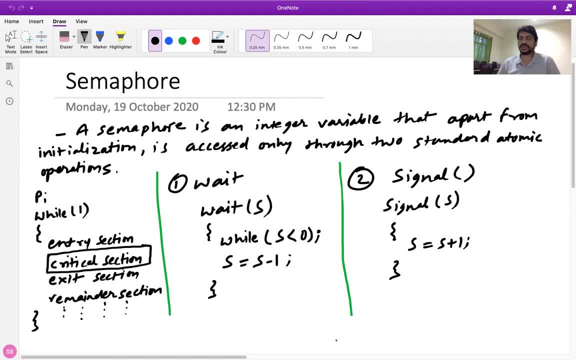 and it is applicable for more than two processes means n number of processes we can use here, and we can use it for the critical section, and for that we use actually semaphore concept. now let's understand what do we mean by semaphore. now, semaphore is an integer variable. 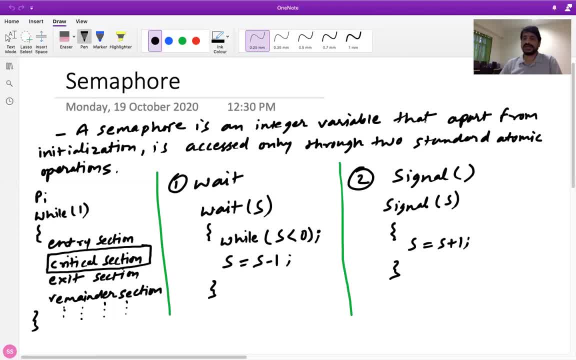 so you can see that semaphore is an integer variable that, apart from initialization, is accepted only through two standard atomic operation. now what will happen is semaphore will be initialized with some value, so a semaphore generally we represent with the variable s, s for semaphore you can take a, you can take b, you can take x, y, z, whatever variable you want to. 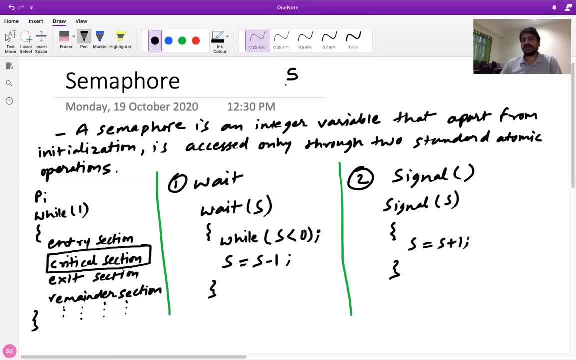 take, you can take it. but to understand the variable type, we say it is a, we represent it with the s. so let's say if s is a semaphore, this semaphore could be initialized with any of the very value. let's say it is initialized with 0 list, as is 1 initialized with any integer we can use. 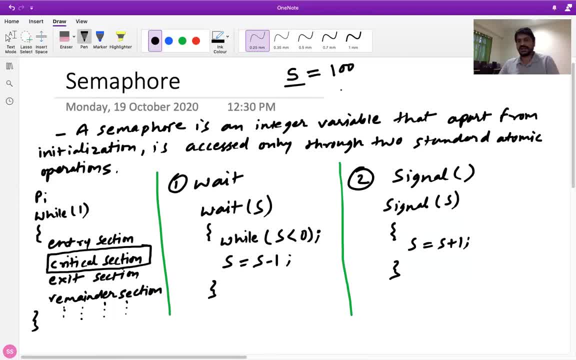 so until initialize with 100. so any integer we can take it to initialize it. but which particular operation will access it? so it will be accessed by standard atomic operation which is called weight and signal. so we have two atomic operation once. one is weight, another is a signal. 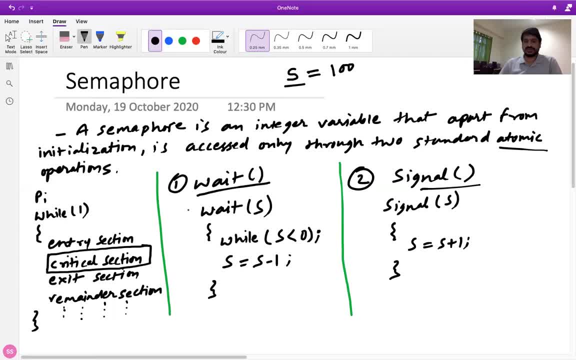 now again it is atomic. one means from here to here, all the instruction will execute. once means in a one cycle. there is no interrupt. from here to here, the execution will done in a single cycle. no interruption could be allowed. now let's see. what do you mean by weight and what do you mean by signal? so once a process want to 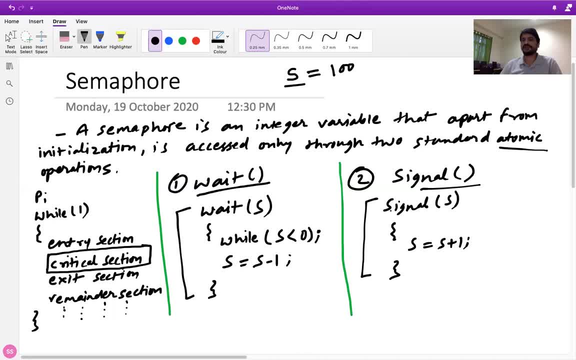 execute the critical section, it has to call the weight function or the weight operation and once the process will get out from the critical section, it will call the signal function. very simple, right? so in this typical, in this typical program, here in this particular box, we have critical section before critical. 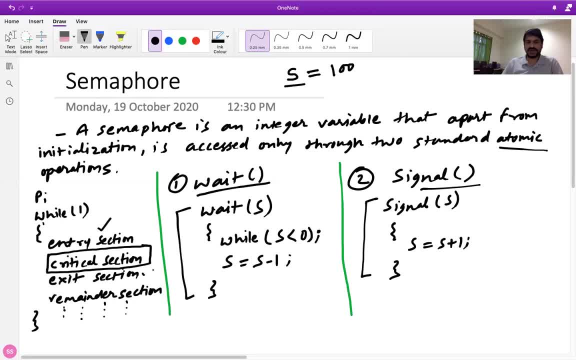 section, we have entry section and after critical section we have exit section. so assume that in the in the entry section we can use weight or we can call the weight function or the weight operation, and in the exit section we can call the signal operation. okay, now about that we'll see shortly. 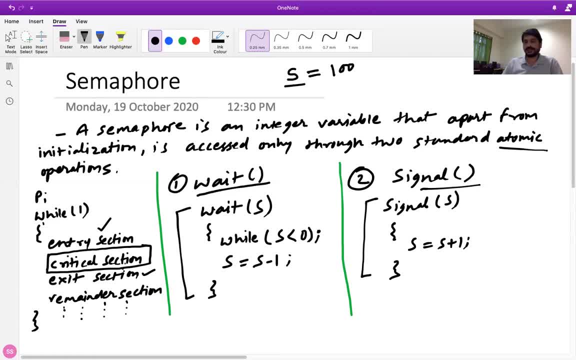 before that, let's try to understand weight and signal now. first you understand signal function. so signal function will take s, what is s as is the integer right semaphore, integer or the semaphore variable. so s value is the weight function. so we will start understand weight and signal function. 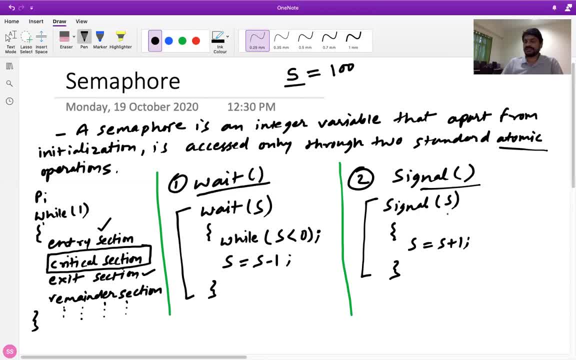 value will put into the signal and whatever the s value is will make it plus 1. so it will just increment the s value to 1, or the sum of 4 to 1. now what weight will do? weight will also do, also take s value, but it will be doing the. 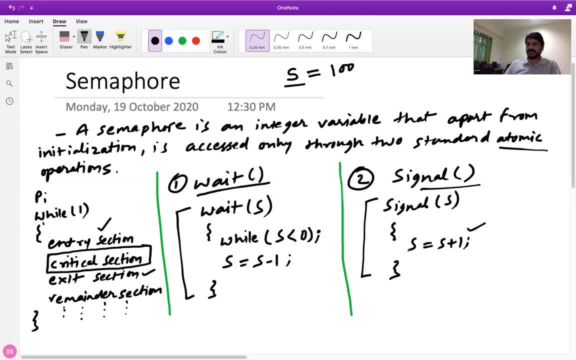 opposite of it: it is incrementing. it is the increment. it is incrementing s value. it is decrementing s value. now this s value will be decremented here, but before that we have a condition to dissatisfied. if condition is satisfied will be in the loop, because here we have a semicolon. so if condition is satisfied, 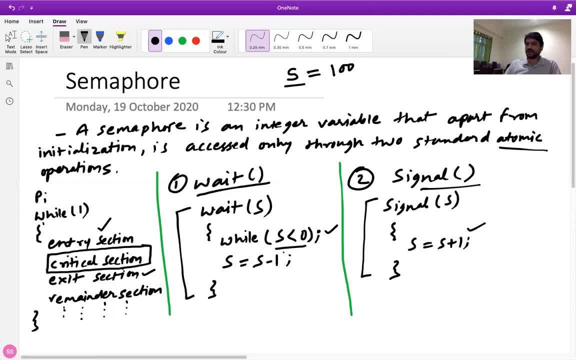 what is the condition? condition is if s is less than 0 or not, or you can say s is less than or equal to less than, or equal to 0 or not. if s is less than or equal to 0, then what will happen? condition is satisfied and will be in the loop. if s is not less than or 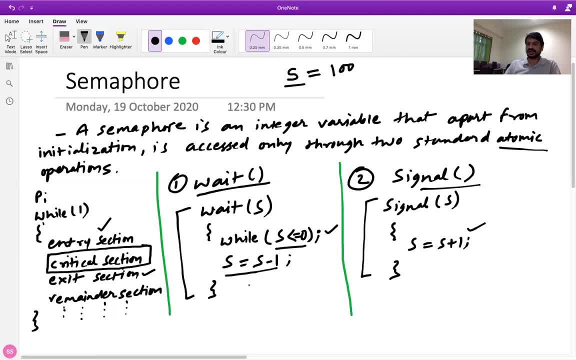 equal to 0, then this particular instruction will be executing, which is s equal to s minus 1. so let's assume that the value of s, the value of s, is 1. so let's assume that the value of s is 1. let's assume that, and there is a process, p1 right? so, as I told you how, 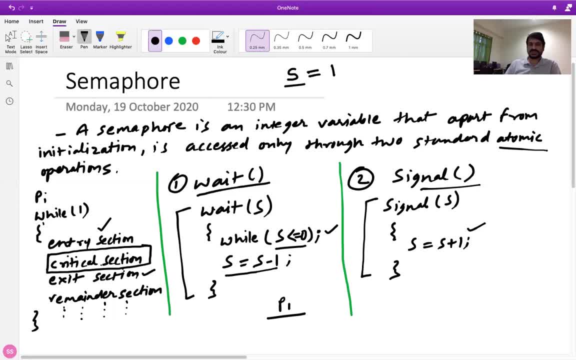 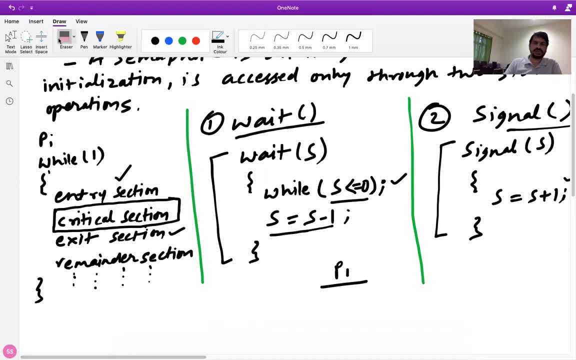 your, your instruction will look like. so here, this is the instruction with the while loop. let's make it to the semaphore that how? if you'll use the semaphore, then how it looked like. so we have the end critical section, but instead of entry section, instead of entry section, we call wait with the 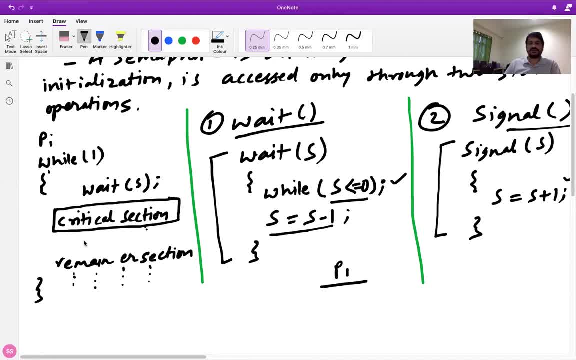 value of s and after that we'll call signal with the value of s and then reminder section is going to be executed, right? so if P 1 is there and P 1 want to execute to the critical section, so the first, what it will have to do even has. 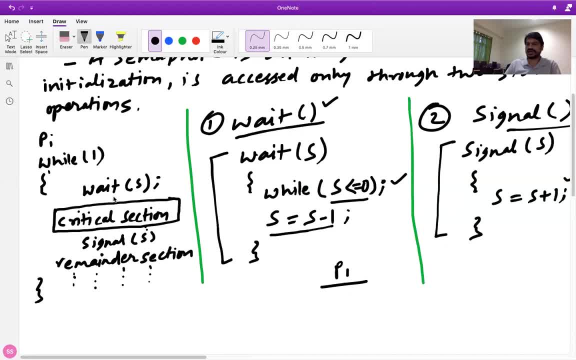 to call the weight function, because this is the entry, and wait will call with s, so it will call a weight with s. what is s value? s value we have taken as 1. now, once it will do that, once it will do that, wait, 1 s is 1, 1 is. 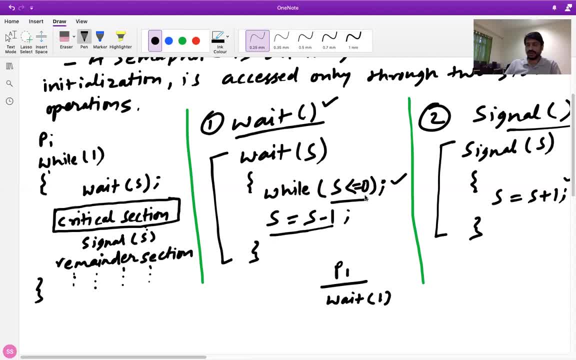 less than equal to 0. is it satisfied? no, it is not satisfied, then we'll go out of the group and we'll execute this, which is s equal to s minus 1. so what is the value right now? and s value was 1. it will become 1 minus 1. it will become 0. so, right now, what is? 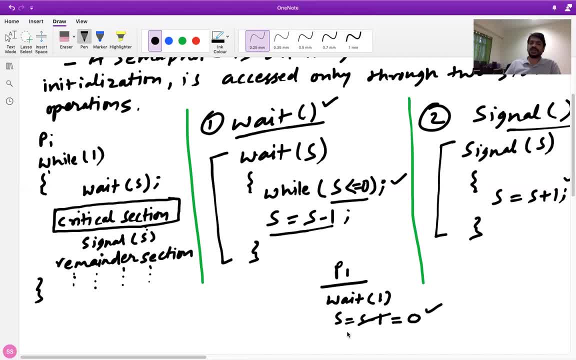 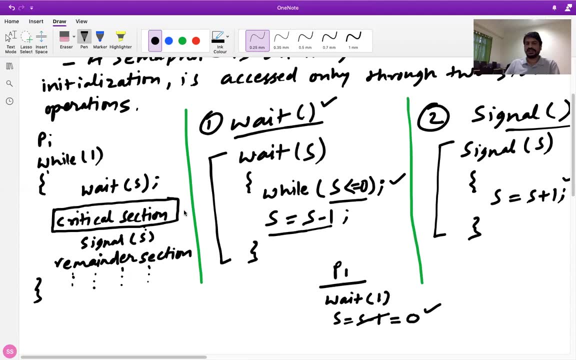 the s value. the s value is 0 now if the s value is 0, it will be. after that it will go to the critical section. once a process in a critical section, it will execute the critical section. once it is getting out, it will call the signal. what? 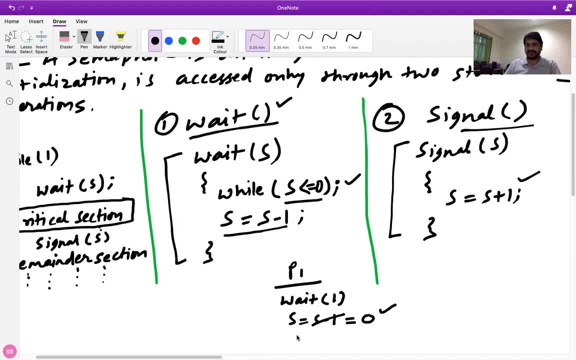 is signal. signal is again s right, so we'll call the signal with the value s. and what is the value in? s is right now 0. we'll assign 0 here as s, and we'll do s equal to s minus s plus 1, so the s value will. 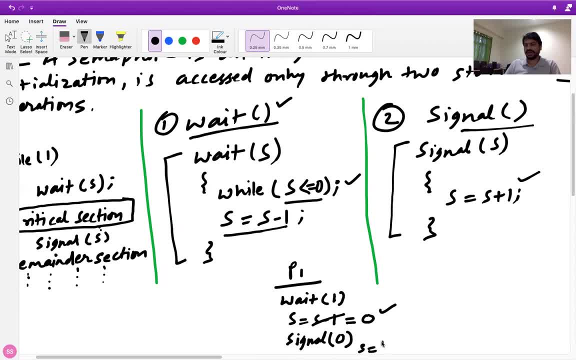 become 0 plus 1, it will be 1 getting. and then let's say p2 is we want to execute, then again p2 also has to do this. it has to wait for the critical section and then after that, once this condition is satisfying the weight, it. 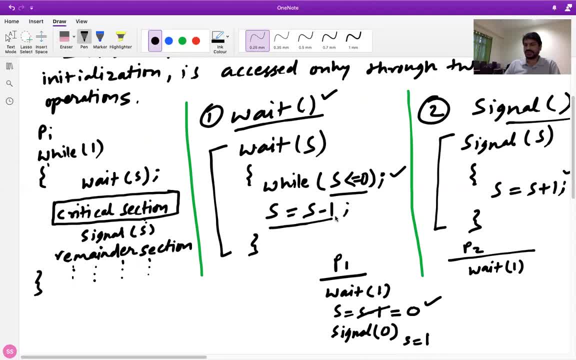 will be call s equal to s minus 1, then it will become s will become 0, then critical section is going to be executed. once it will, coming out of the critical section, signal is going to call. so signal is going to call with s value. what is the? 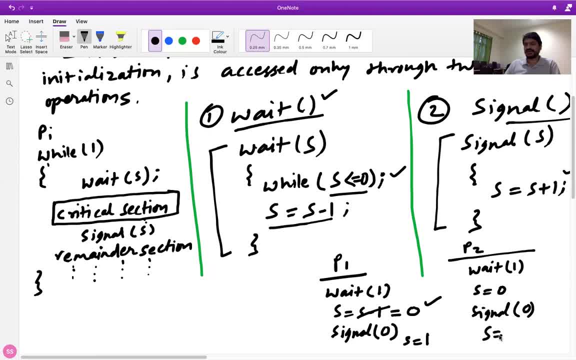 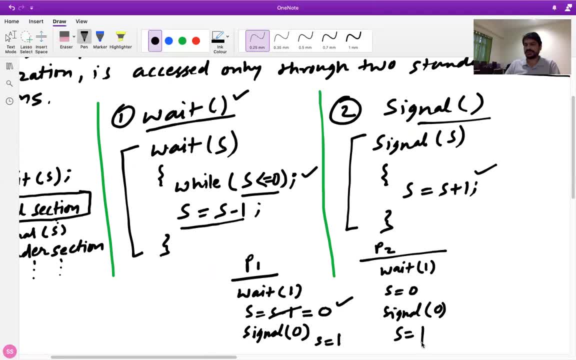 s value. s value is 0, then after that, once this condition is satisfied in the weight, then after that, because it will not have to check any condition, it will just increment s by 1. it will just increment s by 1 in that way, then p3 will come, or maybe p4 will come. 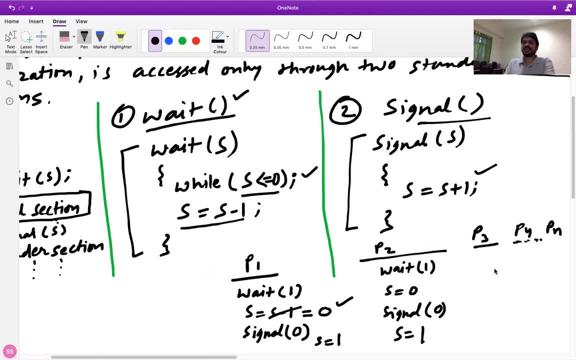 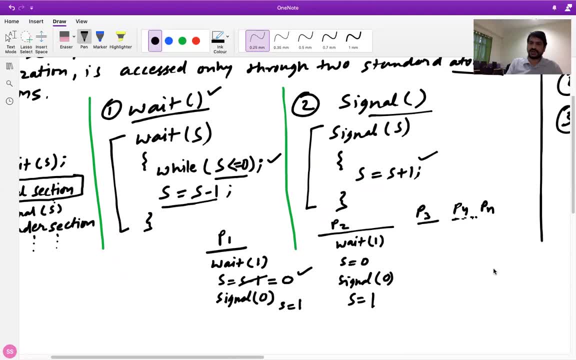 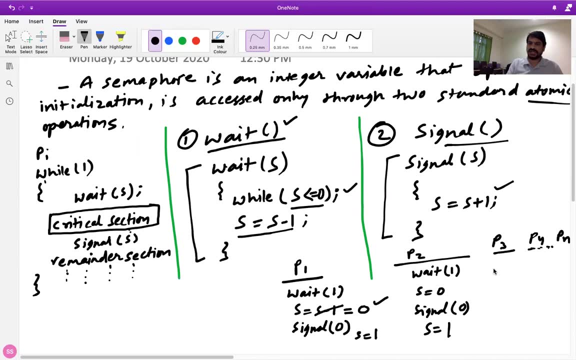 or maybe up to pn, right? so this is how your weight and signal is going to use now. so this is the weight and signal that we are going to use now. so this is the weight and signal and it is the concept of semaphore. now let's talk about the application of 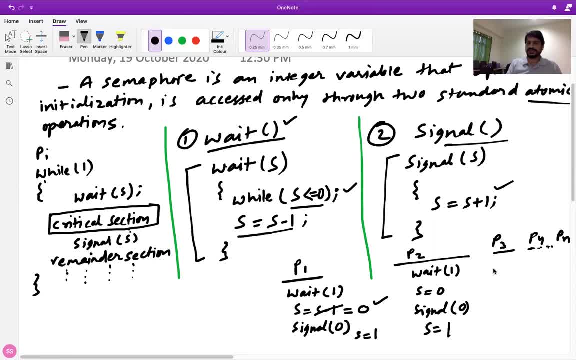 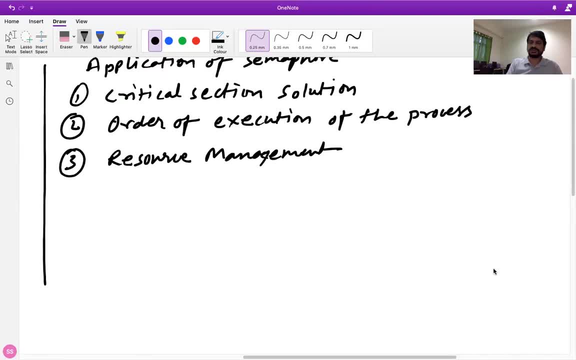 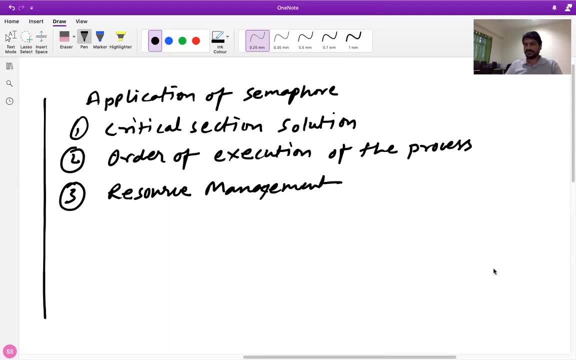 semaphore. we have seen that. what is the usefulness of this? what is weight? weight is signal. right now let's talk about the application of semaphore. so mainly there are three application of semaphore. so the first application is called critical section solution, means we can have a critical section solution here and 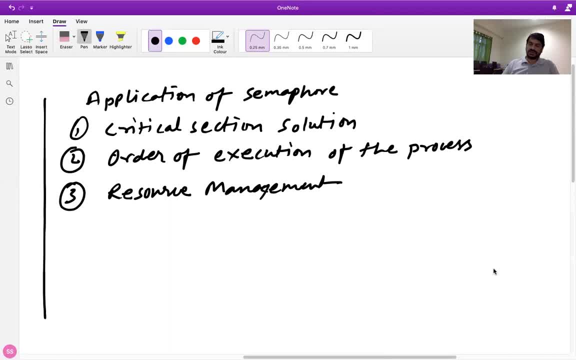 it means that the critical section will be used with the character, with the characteristic mutual exclusion, progress and bounded weight, so the critical section would be achieved. second: order of execution of process. this is the second application- means with the help of the semaphore we can actually order the execution of the process. let's say we have 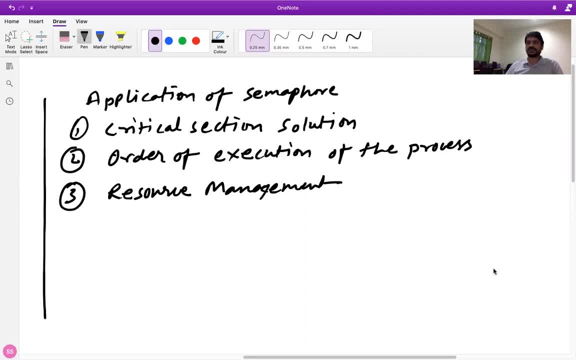 process, p1 to pn. so which process will come execute first and after that? which process will execute after that? which process will execute after that? which process will execute? all these things means the order of the execution of the processes which are available could be done using the semaphore. next application of the semaphore are called resource management. 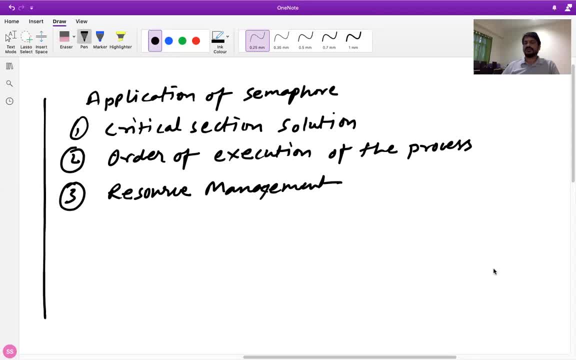 it means that if we have more number of resources and based on the request to that resources, how we can manage it. it means that how we can assign the process to the resources, what the process is required. let's say, a process is required to printer to print, or a process is required a scanner. 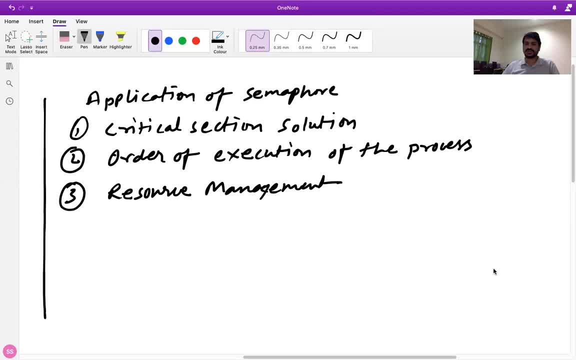 or a process is required, the cpu or a process is required. something else, other resources, so how we can allot it. so the management of the resources could also be done using the semaphore. so mainly semaphore has three main application. first application is critical section. solution means it could. 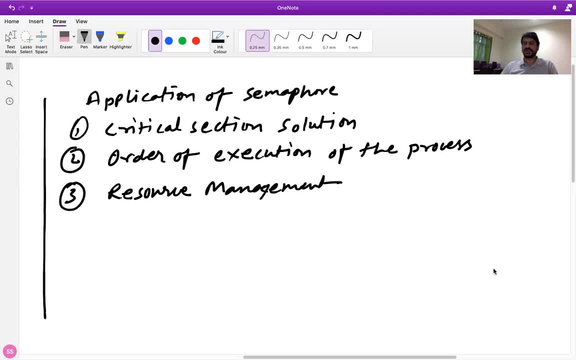 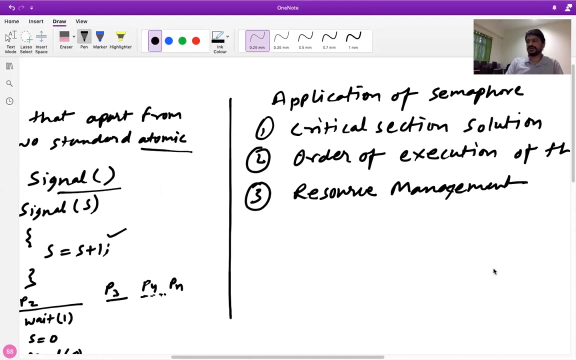 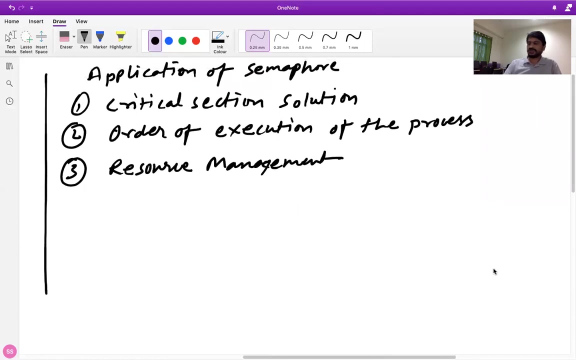 achieve mutual exclusion. progress and when or bounded weight order of execution will be achieved here with the help of semaphore, as well, as resource will be managed very easily with the help of semaphore. so the first solution is called critical section solution. now the critical section solution. we all know that what is a critical section? so critical section is nothing but a part. 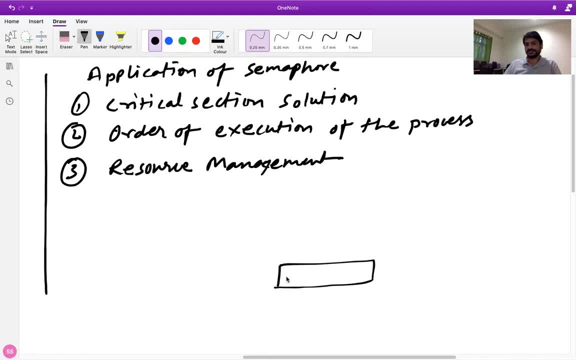 in the code. this is nothing but the part of the code which is subject matter, integration, which is part of the code, which is a a whole thing without any of that. these are just a few examples. so code which is a shared resource between two or more processes. so assume that. 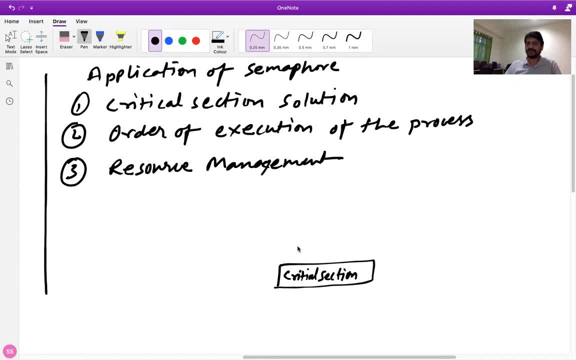 this particular critical resources are here and we have something n number of processes. we have P 1, P 2, P 3, up to n number of processes. and so what is the solution? the semaphore solution is this means: before the critical section, you have to call beat function with the value of s, and after the critical 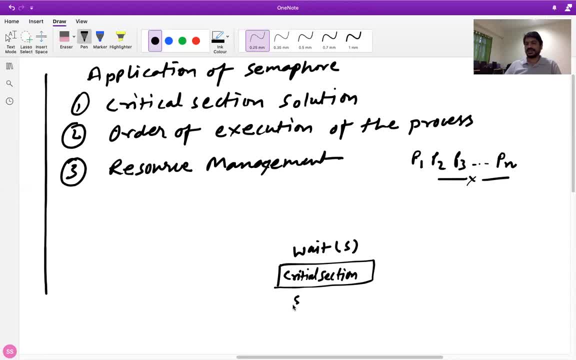 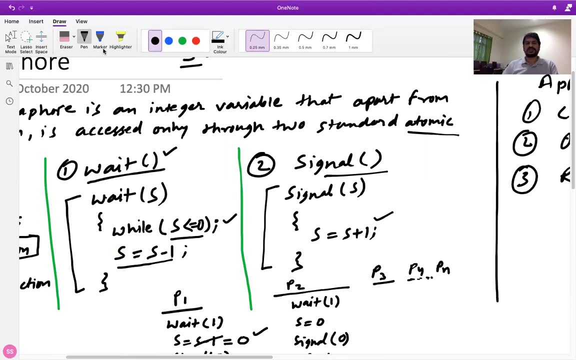 section you have to call signal function or the signal method with s. okay, wait, you already know. this is the definition of weight and this is the definition of signal. so here, the definition of weight is here and the definition of signal is here, right? so this is the definition of weight and this is the definition of. 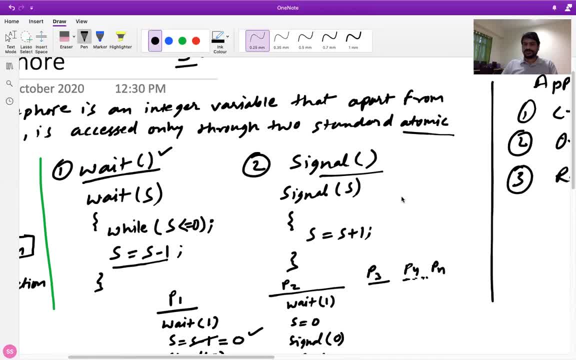 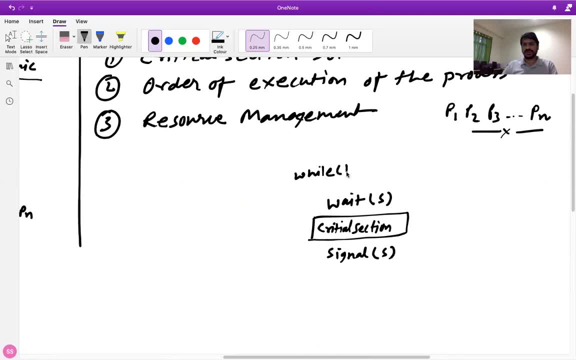 signal that we can use. so this is how your- let's say we, we have a while loop in between these process is going to execute. let's say, here we have the reminder section and let's say this is the whopping wings says that the process is the half of the frontline chains. this is theggs for process. PI means for all the. 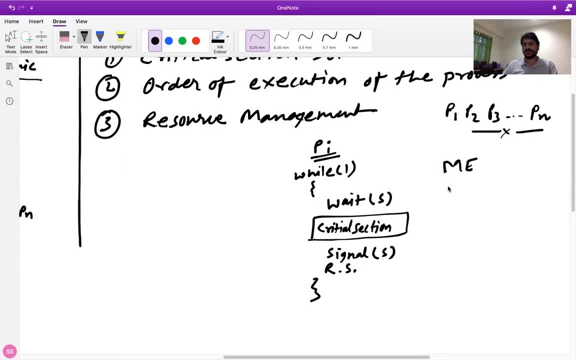 process and this is the code. this let's talk about three most important criteria. first is the mutual exclusion, second leaves progress and the last one is the boundary. I let's see one by one. so the first one is the mutual exclusion. mutual exclusion is one and the other is partial exclusion. then not the case is one by one. two per you's a hundred power toaldo a. 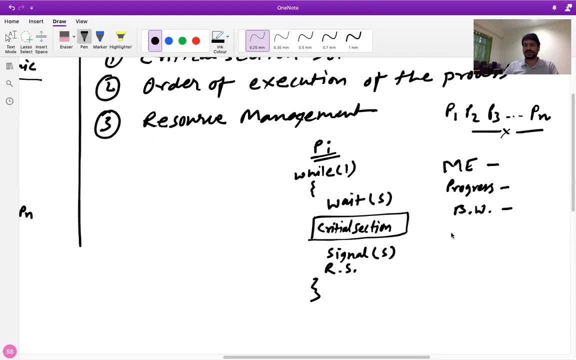 one of the example of the process process is supposed to be this condition: the call, which means all today, means for process thee. class n means if one process is there in the critical section, so will not allow other process to execute into the critical section. let's assume that p1 is already. 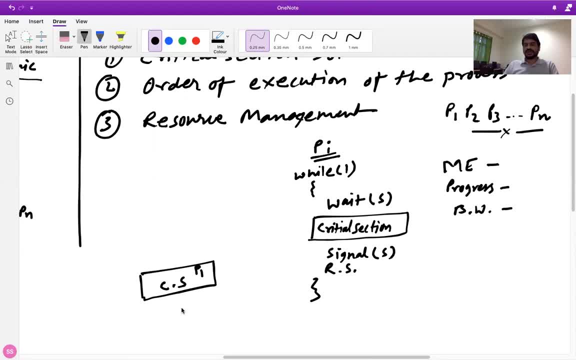 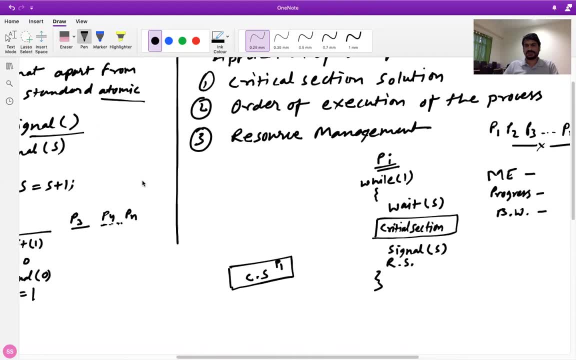 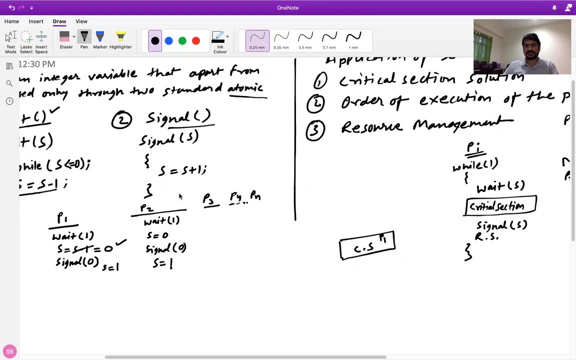 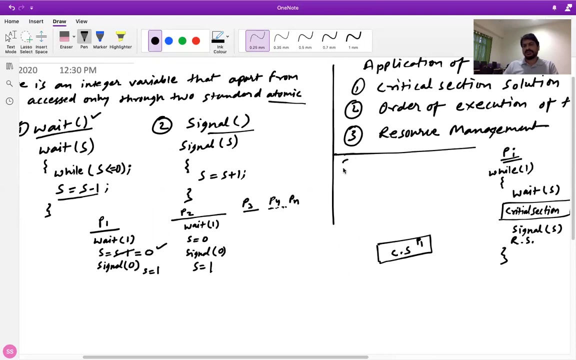 there in the critical section. so for that we'll take from the very beginning. so let's assume that. let's assume that semaphore has a value, one okay. and let's say p1 want to execute into the critical section. so if p1 want to execute, it has to call the. 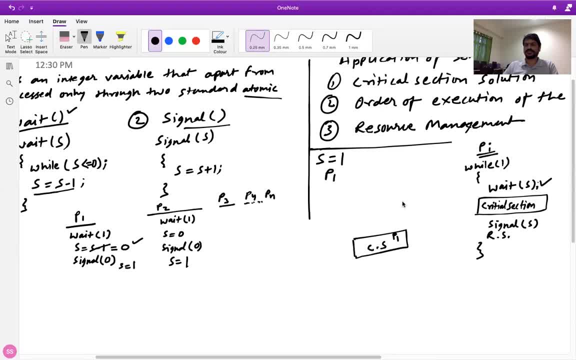 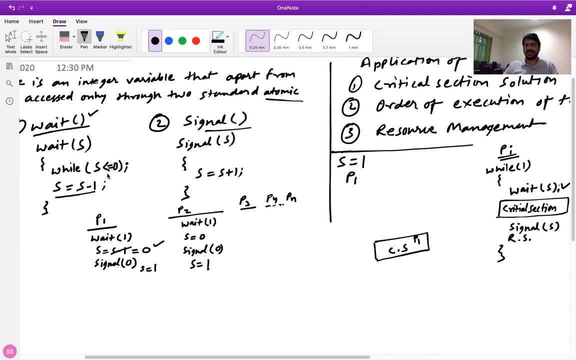 weight function first. so what is weight function? weight function is is having a loop. it says that s value should be less than or equal to zero. you, if yes, it will be in the loop, otherwise it will go out of the loop. so p1 says that, or we'll find out that s value is is zero or less than zero or not. so it 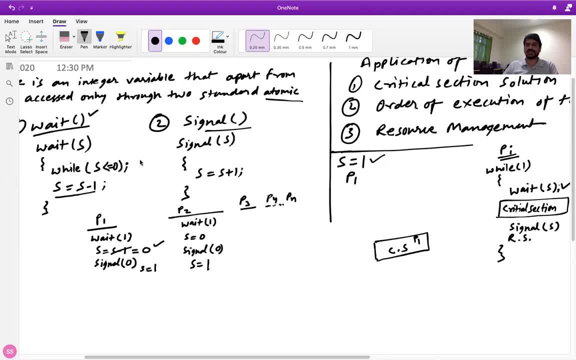 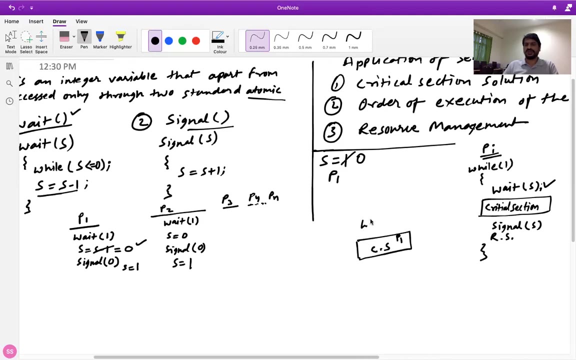 is one. actually, if it is one this is not satisfied, then it will go to the s equal to s minus one. so what is the s value right now? so right now, the s value will be equal to zero. zero, yes, because weight has been executed. now, once the weight will be executed with s, 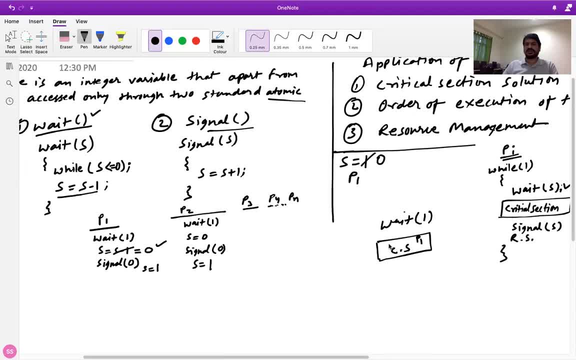 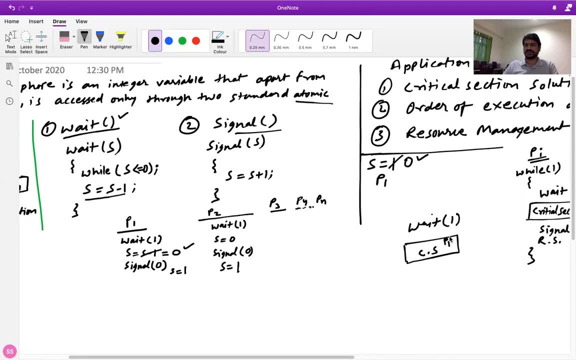 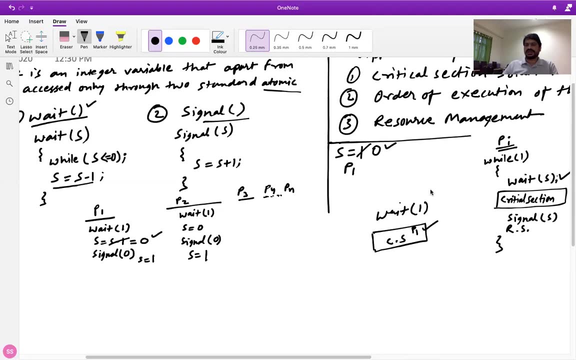 value as one, then what we do is s equal to s minus one. we have done and then, because weight function is already done, it will go to the critical section. let's say p1 is already there in the critical section and p2 come into the picture and p2 want to execute into the critical section. can we allow? 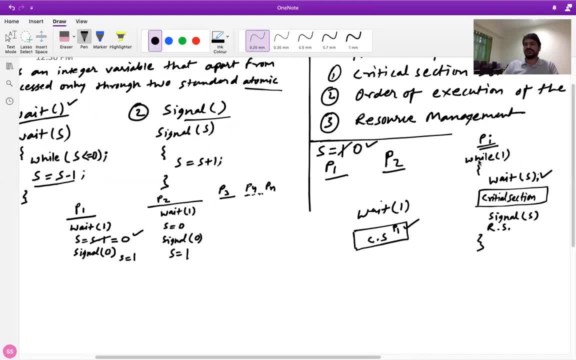 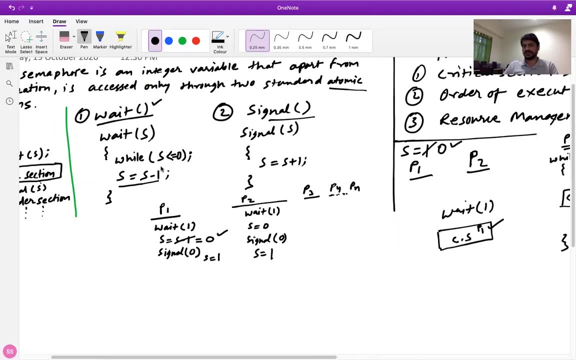 so you see, p2 will also execute the same thing. first, it will execute the weight function. what is weight weight s? what is weight s? here s value s value is zero. so zero will come here, while zero is less than equal to zero. yes, because zero is less than equal to zero. 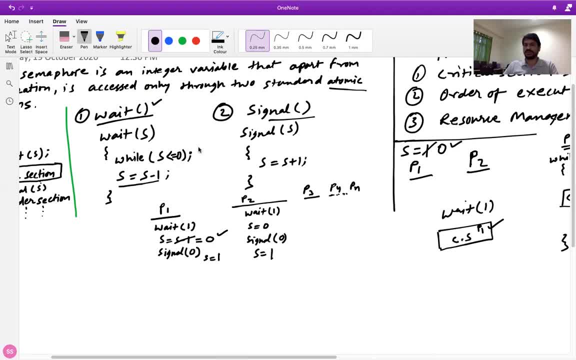 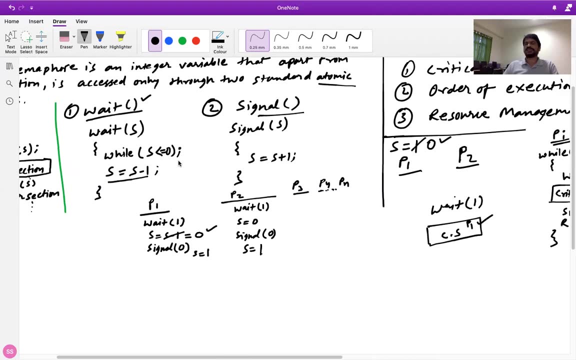 that condition satisfy, then it will be in a loop. so p, p2 will be in a loop and it will never come out. one come till s value is more than zero. so because s value will become more than zero, if p1 will satisfy, all its execution means it will satisfy. 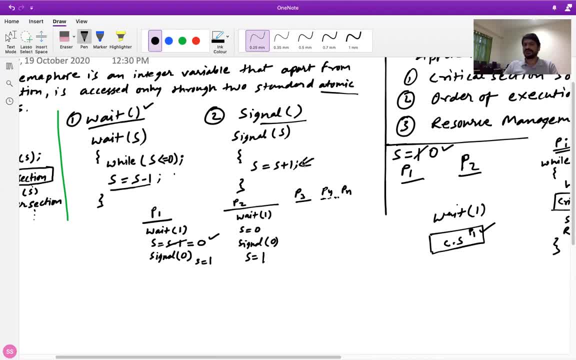 this signal right. so once it will satisfy the signal, then only p1 will get a chance. uh sorry, p2 will get a chance to become. s value is greater than zero because p1 is already in the critical section. p2 will not allow into the critical section, so mutual. 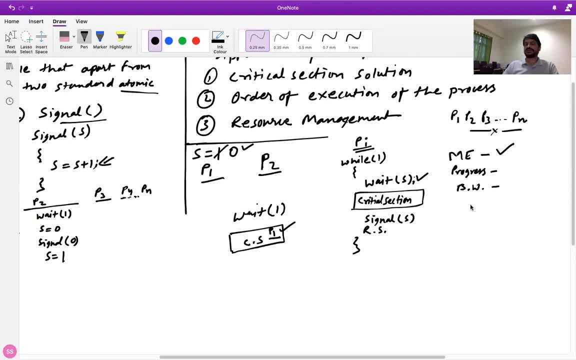 exclusion exists. next is the progress. progress is that if a interested process want to join the critical section, it can join it if critical section is free. so if a process want to go to the critical section, it can go. now you assume that process p1 has executed the critical section going out. 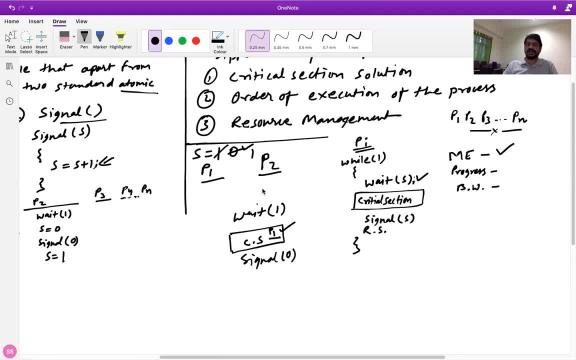 and then this value will be restored to one, and then which process can go. so any of the process can go, there is no problem. let's say p1 is going, so p1 can also can go here and execute the weight and then signal: can p2 go? yes, p2 also can go, because p2 critical section is free and nobody is is stopping that. 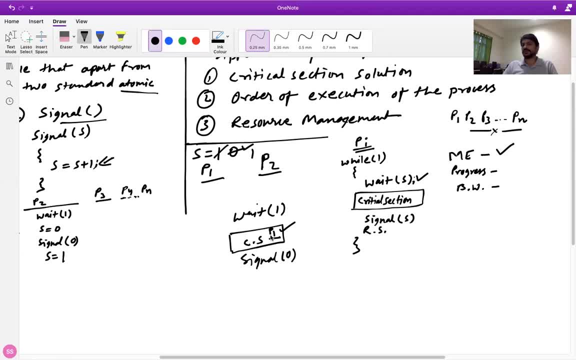 or p3 can go, or people, so any of the process can go. here there is no problem. so any of the process can go into the critical section and the progress achieved. let's see the bounded weight achieved or not. let's say p1 is going into the critical section. 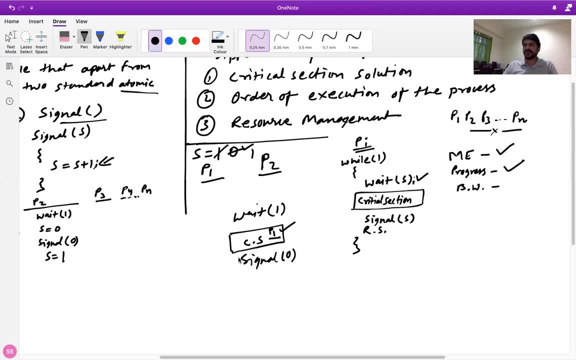 and again, again. p1 will get the chance to go to the critical section, but p2 is waiting to go into the critical section now. here we doesn't have any provision which will tell us that p2 is waiting for the critical section and we can give more priority to p2.